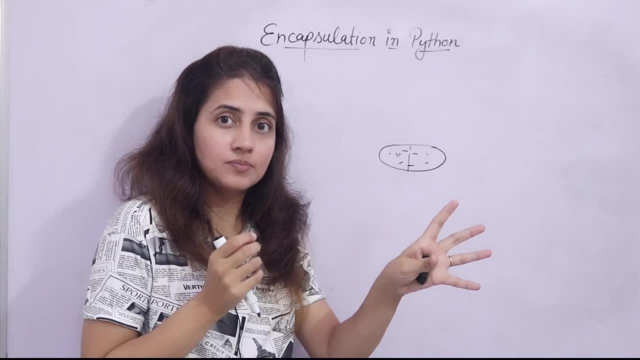 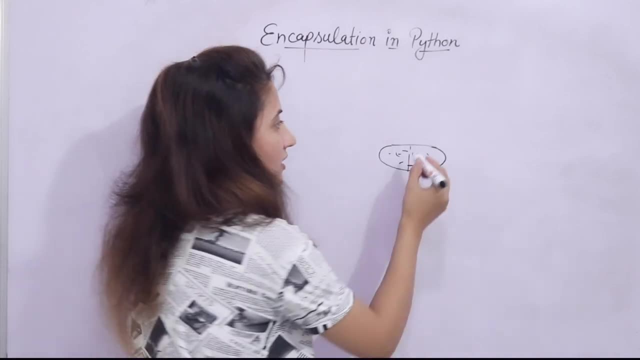 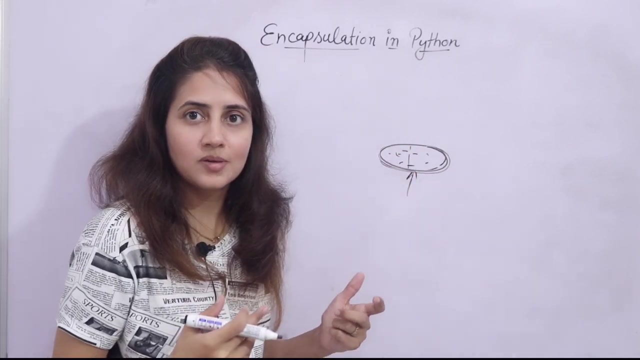 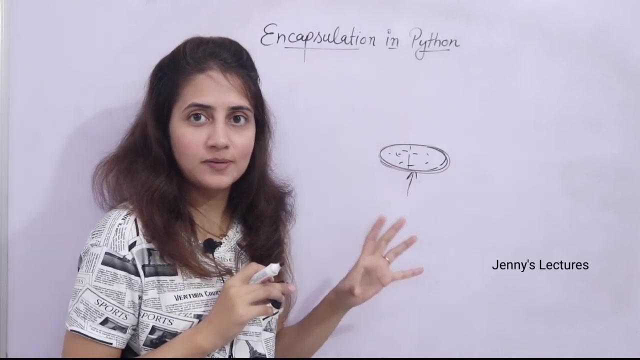 the methods which are acting upon that data into a single unit. that bundling or that wrapping is known as encapsulation. So obviously this is a kind of shield. It is going to protect whatever there inside the capsule From outside world, right. So same in programming also. it is a shield kind of thing. right, That is. 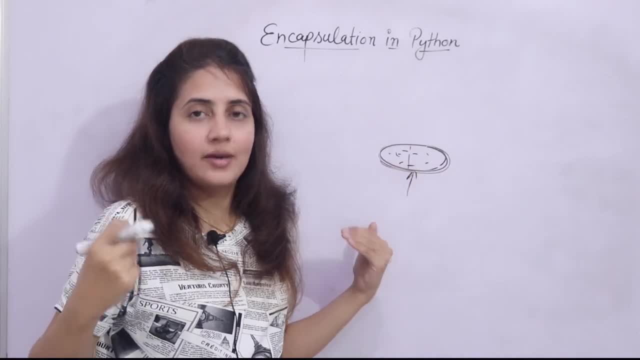 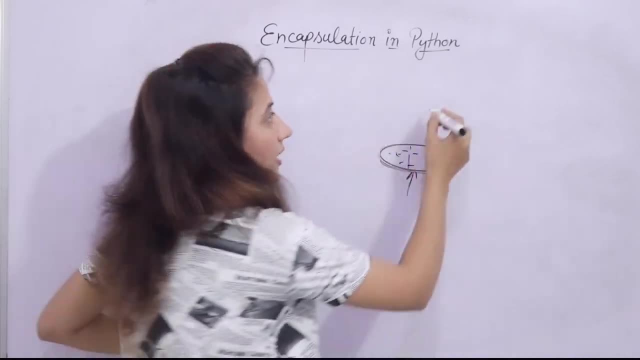 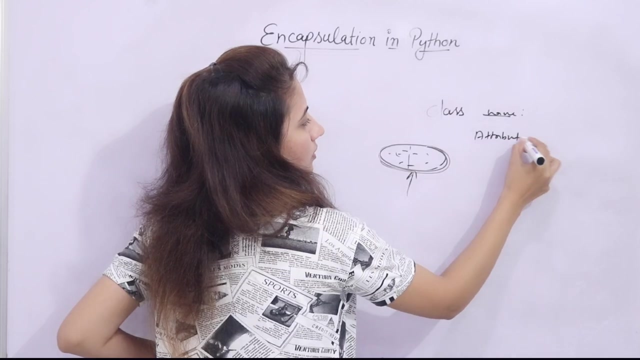 going to protect our data and our method from outside world. Now how? That I'll show you right. So now, basically, if I say, like, if you are defining a class, then what is there in a class Class? here you will have a class name, then some attributes and methods. 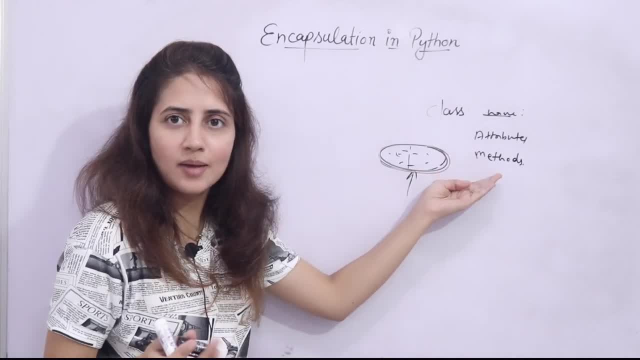 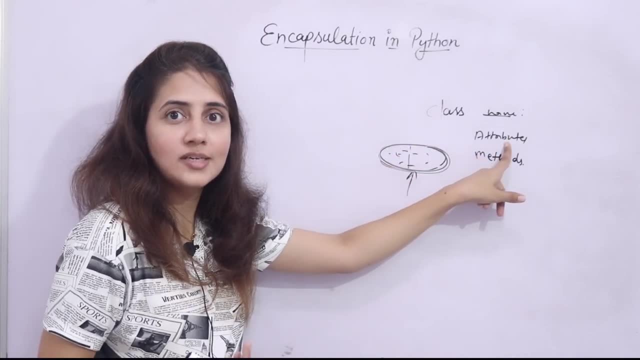 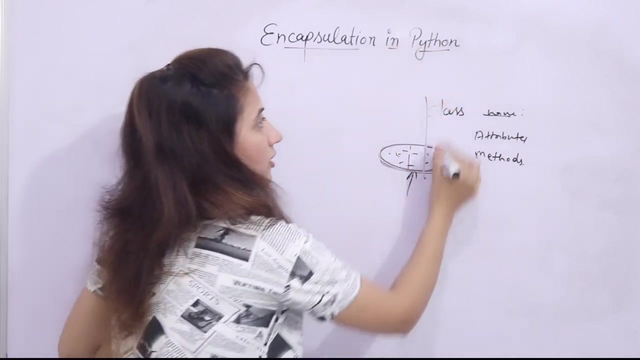 This is class. So this is just an example of encapsulation, Simplest example, Because in class we are having some attributes of the class, or you can say the data of the class, or the member data, members of the class, as well as the methods in the single unit, right. So this is, you can say: 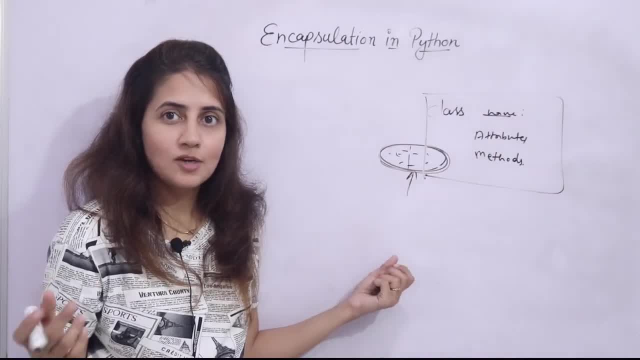 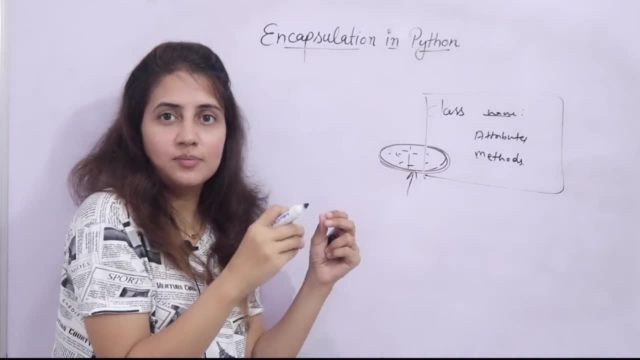 a capsule or this is what: nothing but encapsulation. So, like in real world, we have this kind of capsule And so it's not easy to open that capsule right? Or maybe if something is there in a single unit, then it's not easy to open that capsule. So we have a lot of 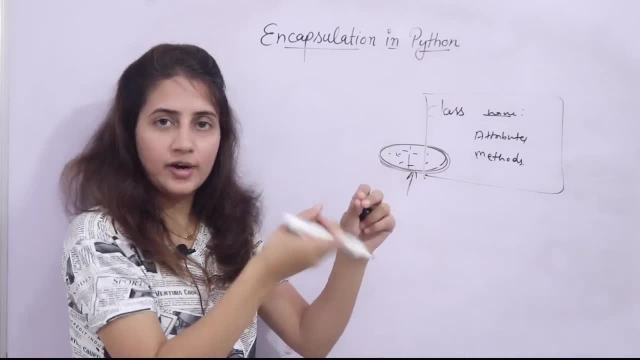 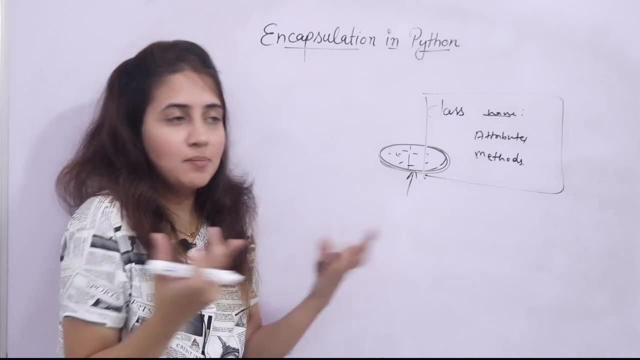 processes, like in previous example. we have discussed X specifiers. So that thing you will put in a locker, you have a lock and you have a key. But in programming obviously we are not having any proper lock or any proper key right. So there are simply some name. 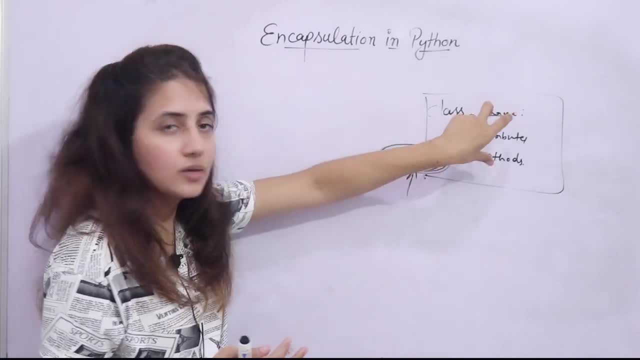 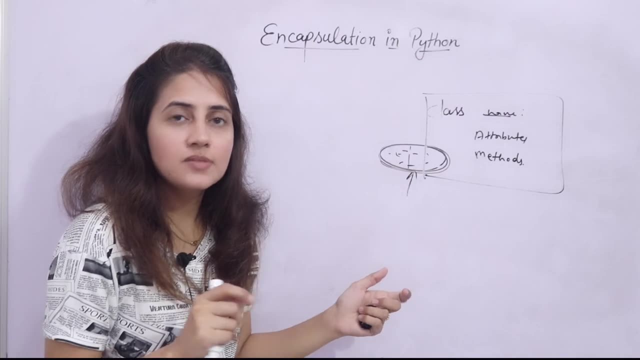 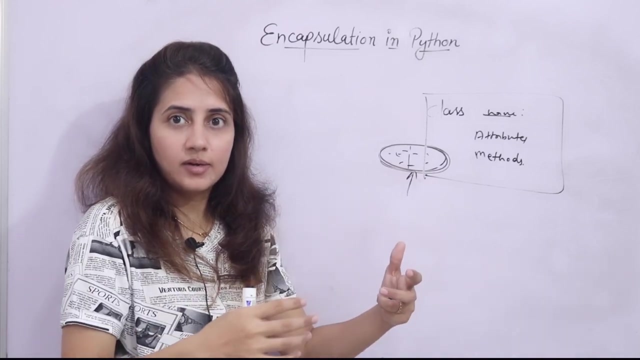 conventions of notification or this kind of thing. right. So here you are going to achieve encapsulation, or you are going to see encapsulation is wrapping up of these things into single unit, also known as data hiding. It protects our data. it hides the data right As well as the 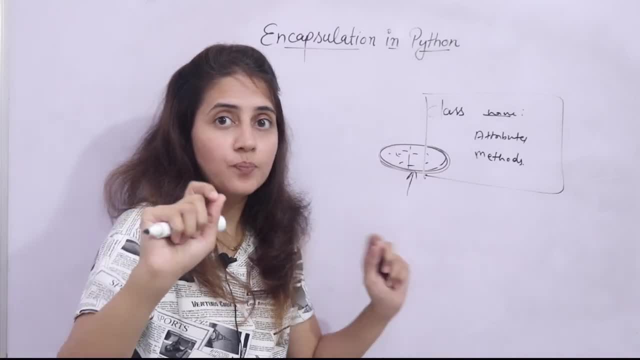 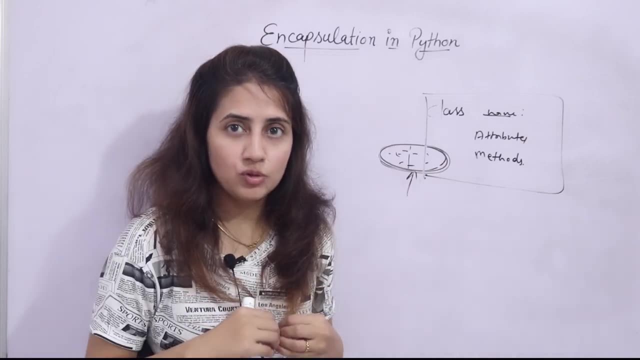 implementation detail from the user: See in abstraction. I have told you abstraction is basically a process of finding out which functionality is shown to the user and which is to be hidden from the user right. But actual hiding is done with the help of this thing. 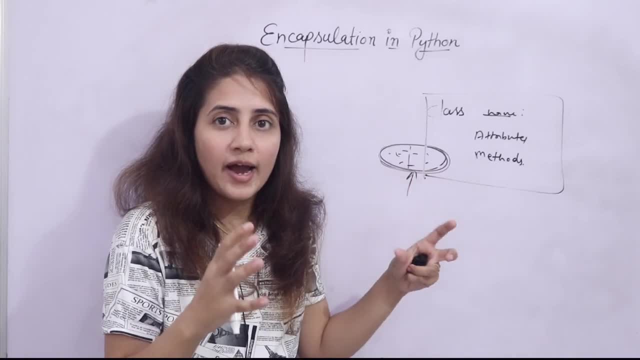 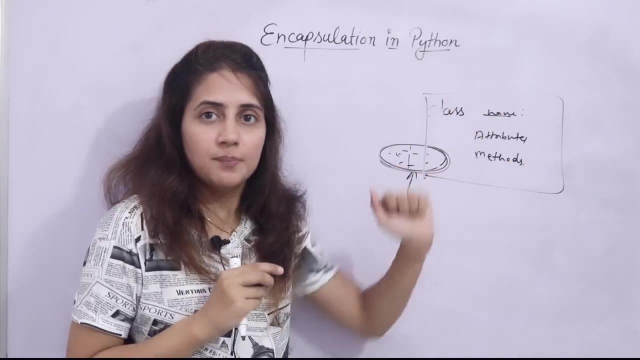 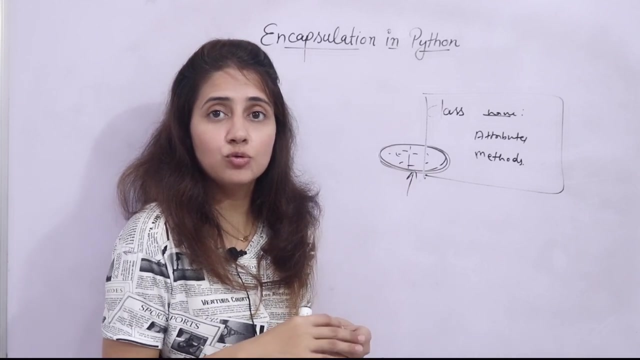 encapsulation. Now how we are going to hide using XS specifier And XS specifier public-private, protected. that thing we have discussed in previous video, right? So encapsulation is also known as data hiding. So I want to hide some data. Then you just declare that. 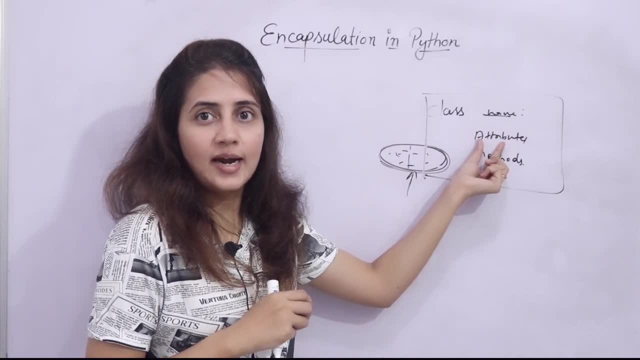 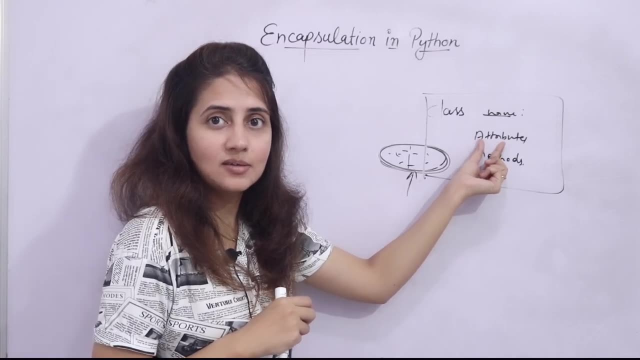 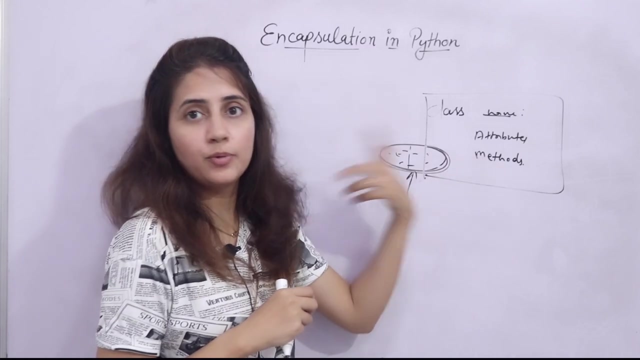 attribute, Suppose student age. I want to hide that age, Right, So I just declare that age variable private. That's it. Or I want to hide some method from outside the world. that also method we can do. We can make that method private or either protected Subscribe. 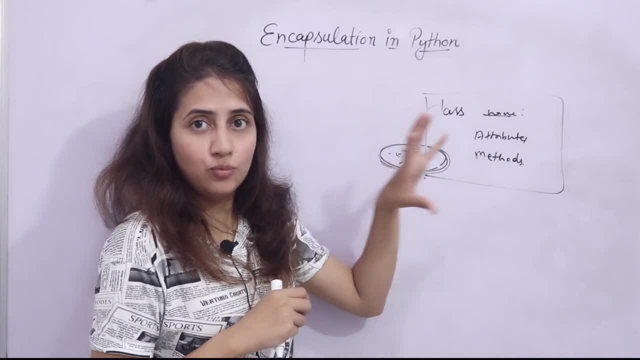 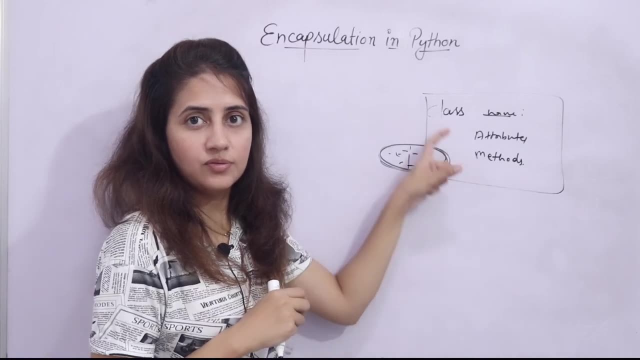 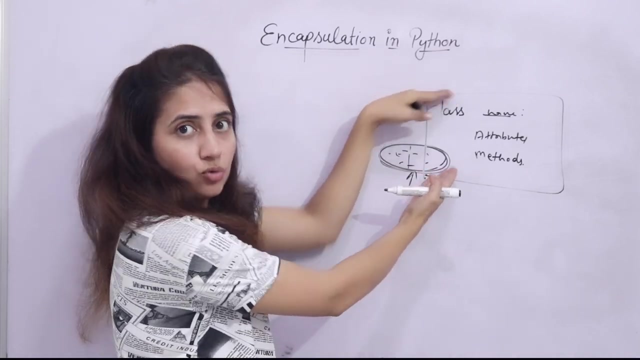 to my channel, right, so in, if you make it protected, then drive the class you know can access those protected attributes and methods. but if a method or in a way attribute is private, then that we can use only inside the class, not outside the class. yes, we. 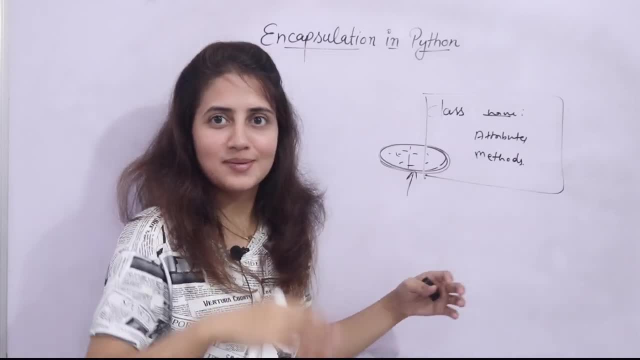 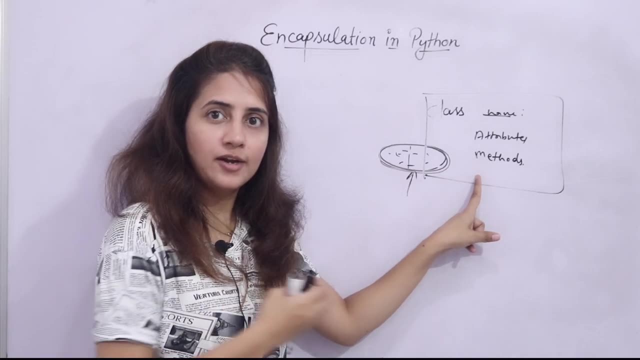 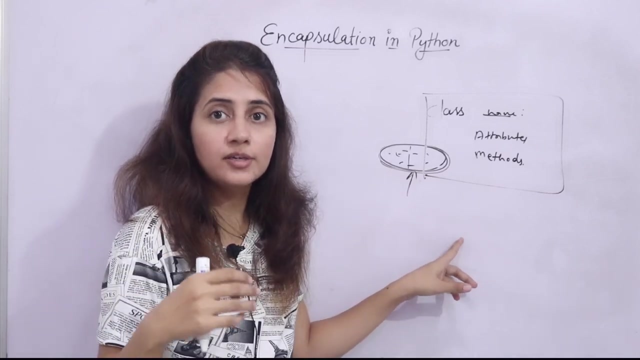 can? we can access private methods and attributes outside of the class. there are basically three methods. first, just create public method within the class only and using that we can access private methods and attributes. second thing, using name mangling. and third thing, using getter and setter methods. so 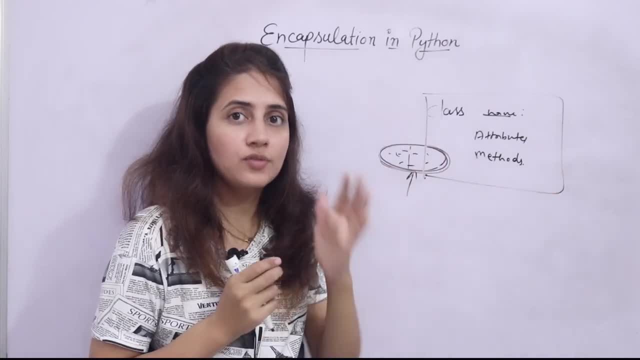 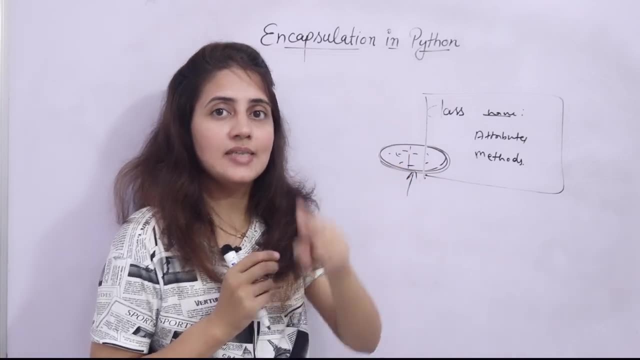 first two technique we have discussed in previous video. please watch that video first. right, that's very important to get encapsulation. now third method: using getters and setter method, how you can achieve encapsulation, that thing I'll show you practically in this video. but I hope now the basics of encapsulation. 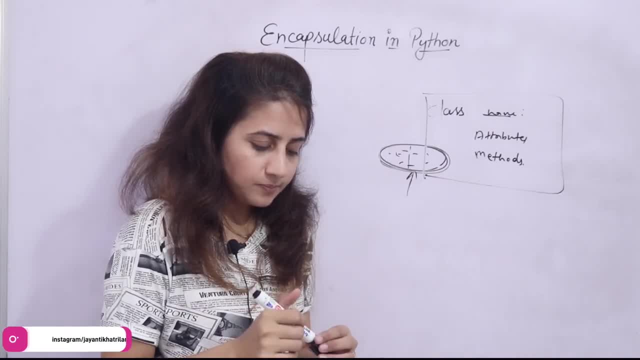 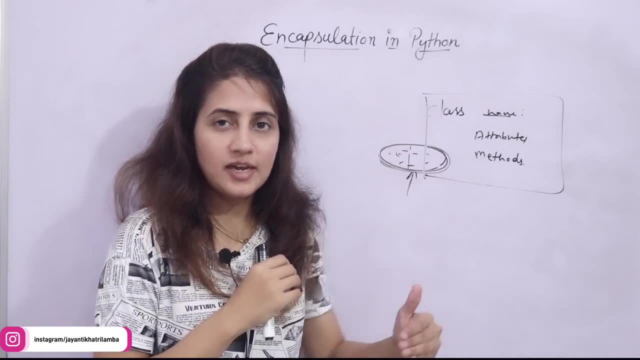 what is encapsulation is clear to you guys. you can see that I am showing you the basics of encapsulation. what is encapsulation is clear to you guys, right? so if I say what are advantages, or let me just show you that practical example and at last we will just summarize this thing and I will show you. 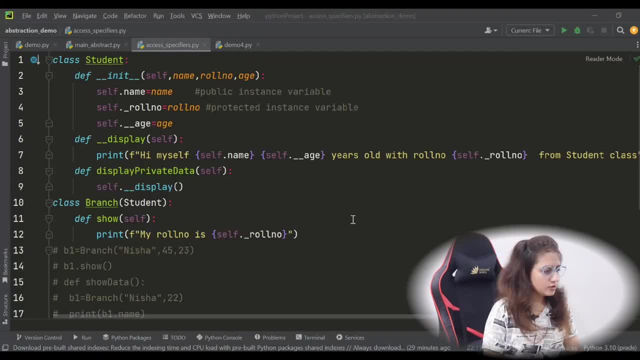 I will tell you the advantages of encapsulation, right, okay? so see, this was the example you have taken in previous video when we're discussing. it's a specifier, public, private and protected, because obviously using these specifier only we can achieve encapsulation. we can hide our data, right, or you can say not. 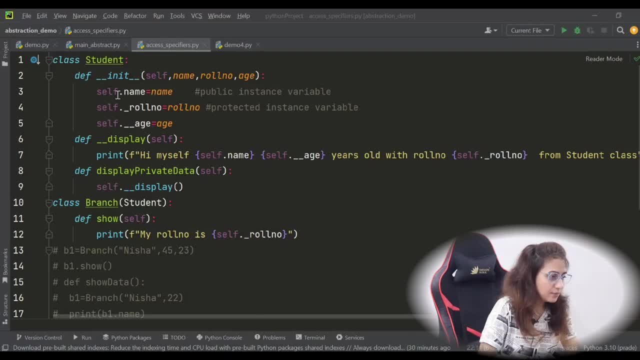 only the data are methods as well as we can hide our data, we can hide our data right, like this example you have taken. this name is public, this one is protected. if the this is a prefix to the one and one underscore that is protected and this age is private, private instance variable, so it is prefix with double underscore. 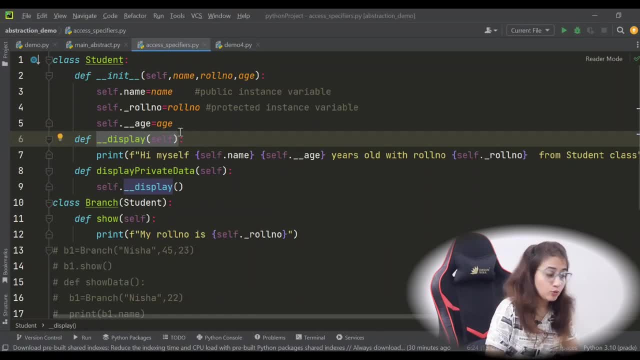 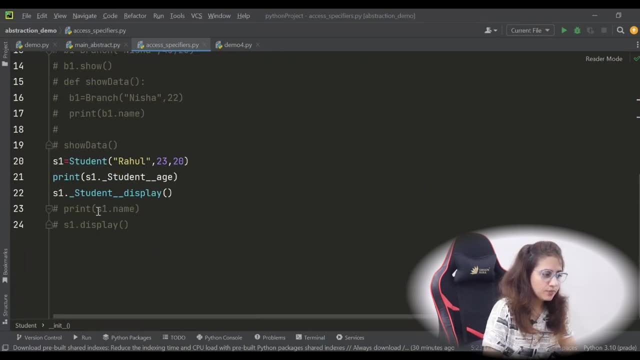 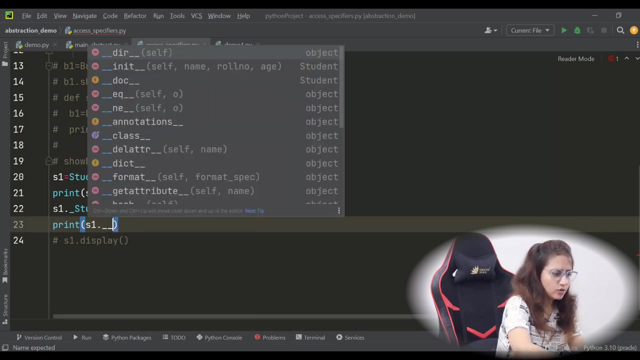 and we have a private method as well as right. so if you want to access this private attribute outside of the class and directly with the help of this, we cannot access. if you want to print directly with the help of like yes, so this one, and underscore- underscore age. I want to print age, so it will give error. 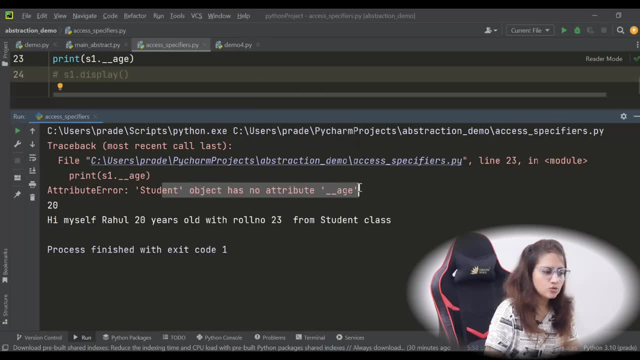 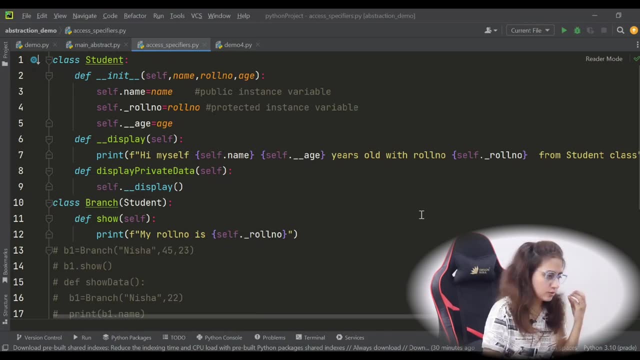 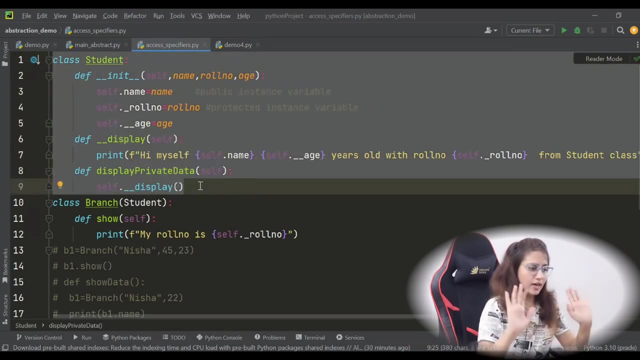 see attribute error. student object has no attribute age because outside of the class we cannot access private. if it is a private method or private attribute within the class means this area is within the class, only only this area, this object we are creating outside of the class. so that is. 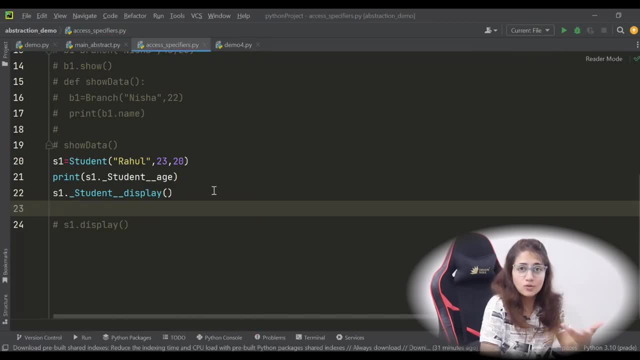 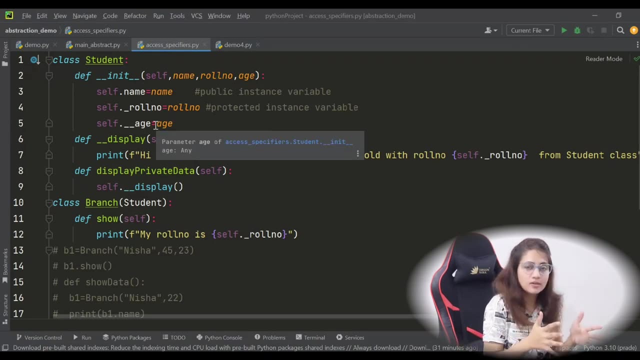 why we are not able to access this thing right. so this is obviously: we are hiding our data, we are protecting our data from public access. we are restricting the access to our data, which is very. maybe some sensitive data we have. in your class it's just a simple program, but in industry, when you are 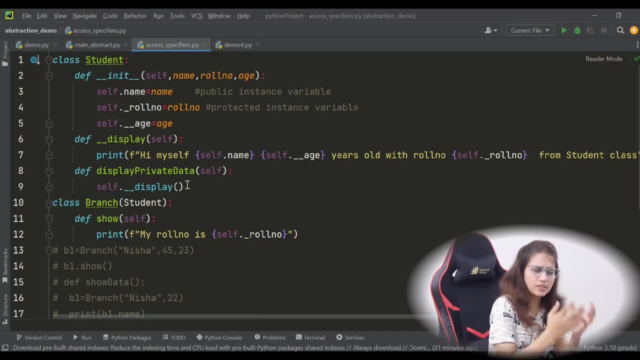 working on project, then definitely there must be some sensitive information in that project so that we are going to declare that thing as private. okay, now how you can access this private project- private kind of thing either- you can use first method is using public method. you can access this thing. see this display. private data is public method. so here I'm. 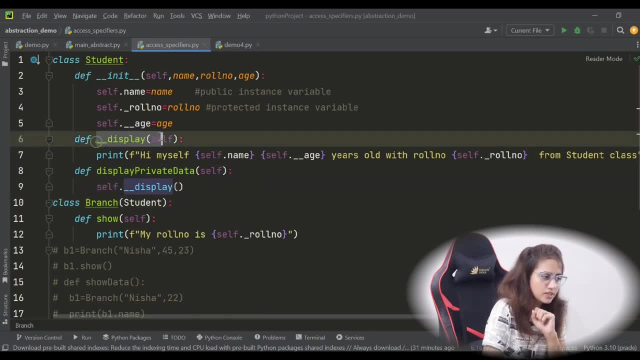 just calling this. this display method is private, so directly we cannot access outside of the class, but within this public method we can access. we can call this method. so have underscore, underscore display and within this display I am accessing age. that is fine, now I can call out. 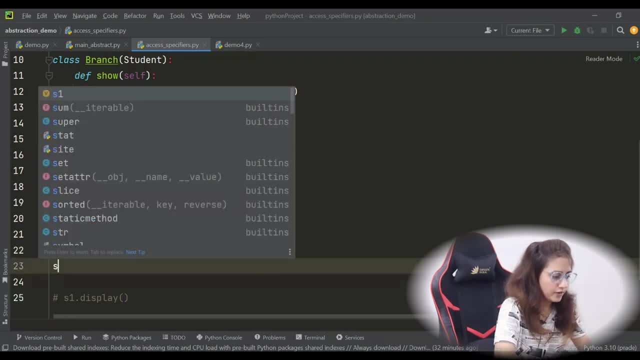 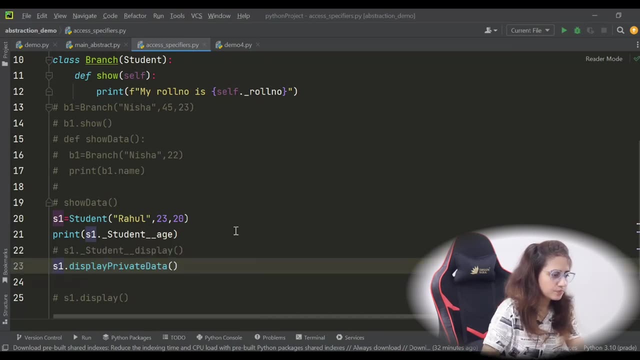 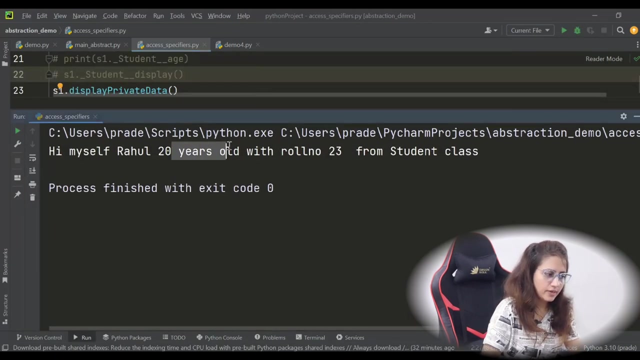 outside of the class. this display private data right. so if I call like s1 dot display private data, then we can access. let let me just comment out this thing. see now Rahul, age and roll number 23 from student class right. like this you can access. second thing: how you can access private data using name mangling. 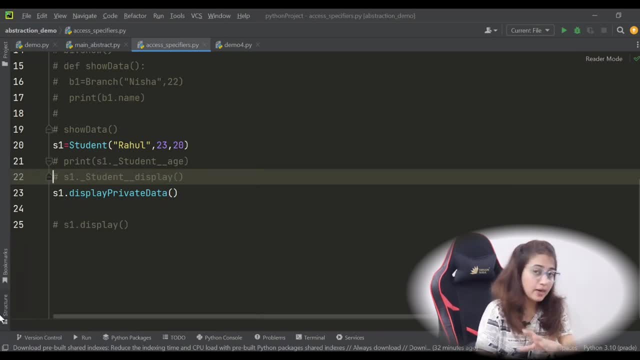 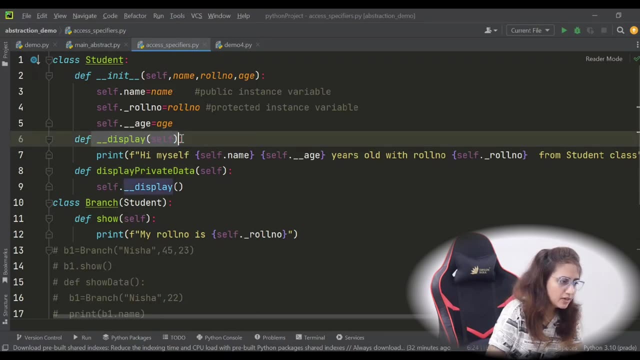 so that also we have discussed in last video: using DIR you can do name mangling and how to access name mangling type of thing. this is the example. see, if you want to call this display method, because this is private, directly you can call, but using name mangling we can call, so name. 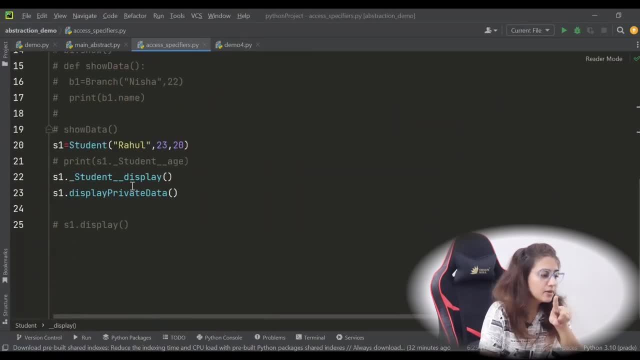 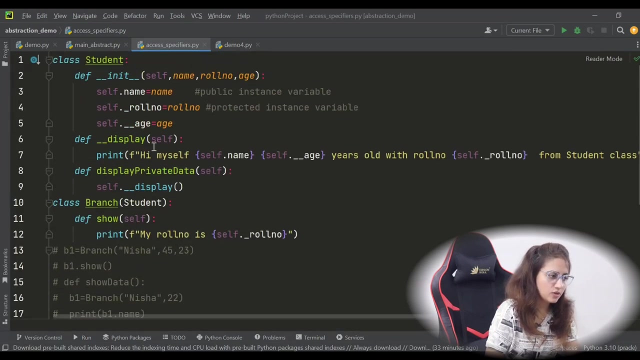 mangling what you have to do: first underscore, then class name, then private data or private attribute name or private method name. this is fine. now this display will work. now. let me just comment out this thing. let's run this now. see, this display is working right, this function. or if you want to access this age, that is also fine. 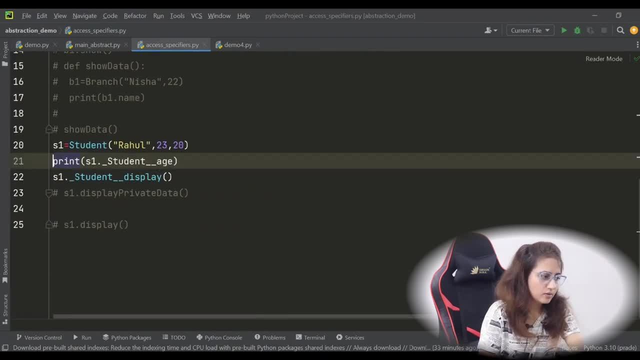 we have see using name mangling the object name dot underscore class, name underscore underscore age. it is fine. third thing is now, using getter and setter method, we can access private kind of thing now. basically, if I would say this is the you know best process, using getters and setters method, to implement. 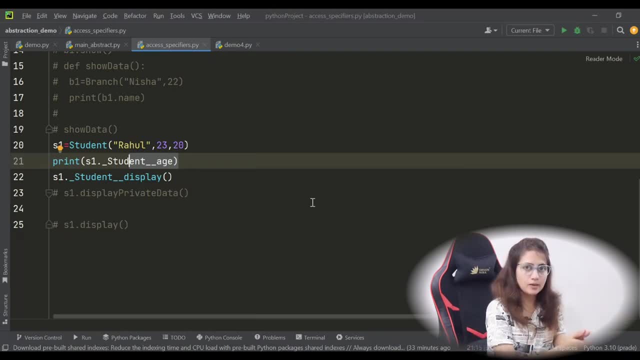 complete encapsulation in your program, right? because, see, we can access private data outside of the class. so in Python there is no such mechanism to completely restrict the excess of private data outside of the class. it's flexible right. it is the responsibility of a good programmer to. 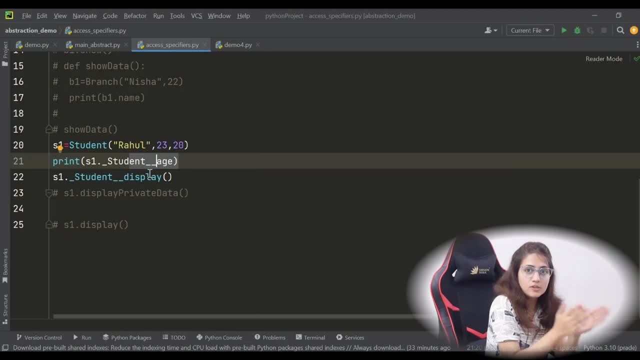 do not touch private and protected members outside of the class. do not modify these thing outside of the class. I can modify this private date outside of the class to modify like this age. then simply you have to access like this and equal to now age. i just want. 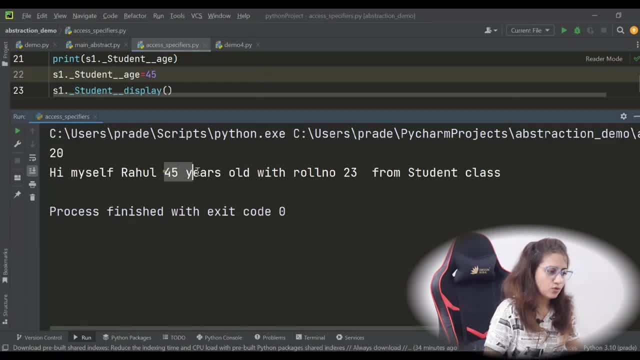 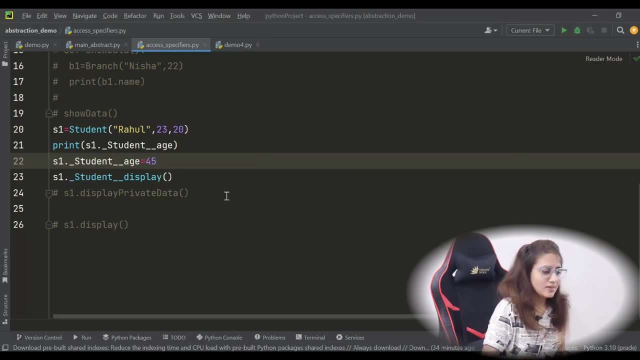 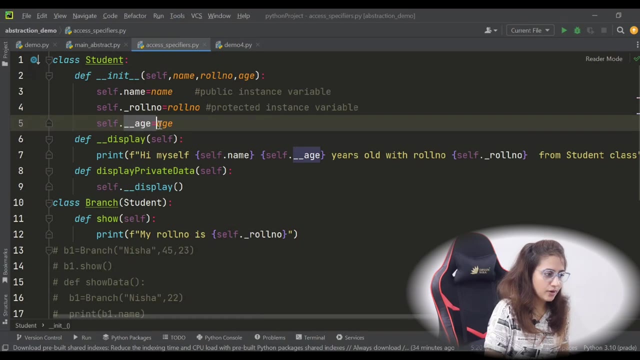 to set 45. let's run this and see 45 year old so i can modify the state outside of the class. now what is the use of this private kind of thing, right? so obviously, if something you have seen, if you are working in a team on a in a company, then if you have seen in a class, you have private. 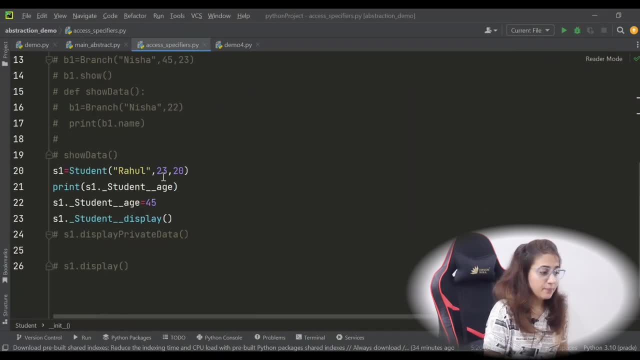 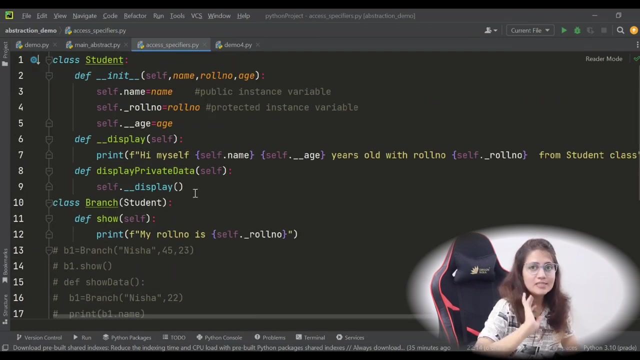 thing- private attribute, underscore, underscore- age- then better not to touch this outside of the class, better not to modify this. it is your responsibility- these are, you can say manners or these are ethics- not to touch these things outside of the class. so always use getters and setters methods. now, getter method is to access the private data and setter method is 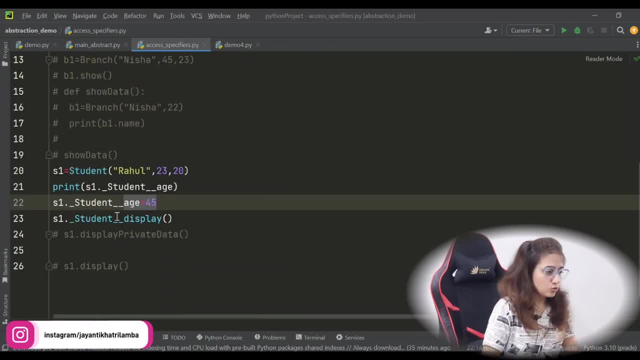 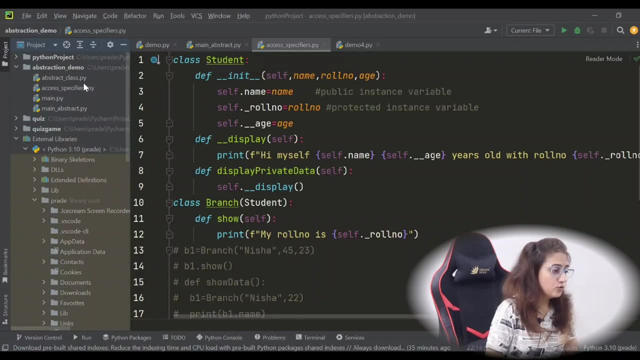 to set or to modify the values, right? so, rather than modifying, find this thing outside of the class. okay, let's create a new project, sorry, new file in abstraction, demo only. and i'm creating encapsulation demo dot py. and let's just copy paste the previous code as: 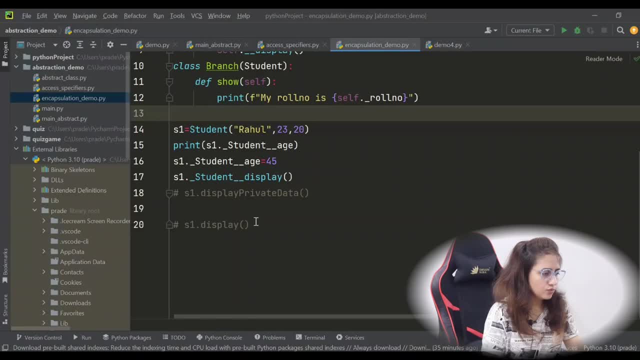 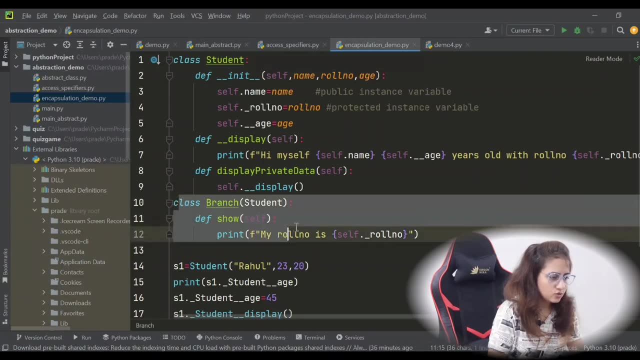 it is. let me just remove first of all something here. right, so we have this class. right, this is drive class. so drive class is basically comes into picture when you are dealing with protected data and in inheritance. basically, if you want that, your drive class can access the data only. 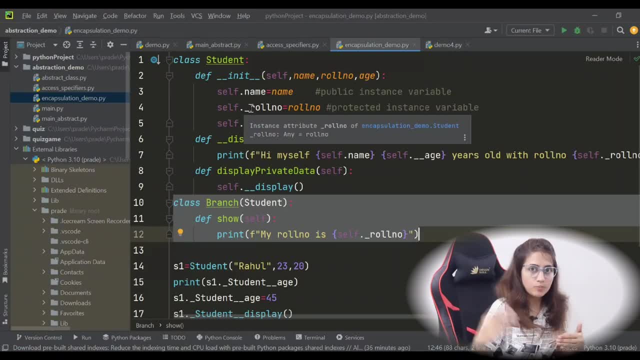 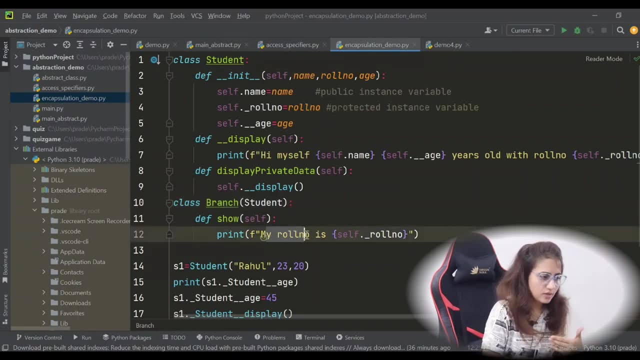 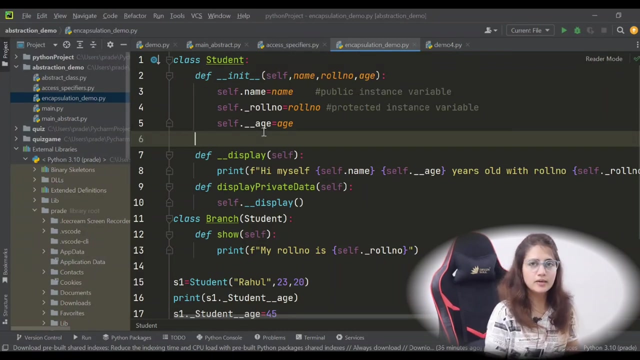 drive class can access the data, not public member, not public person. then just declare that thing as protected. so this roll number this drive class can access. see here, directly i can access selfroll number because this is drive class from student class, right, okay, okay, so now okay, let's use getters and setters method. suppose using getter, using get method, i want to. 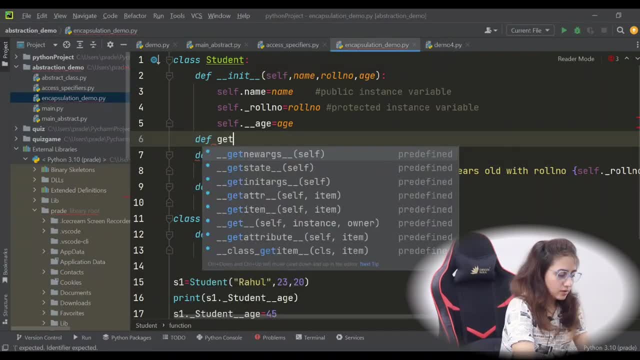 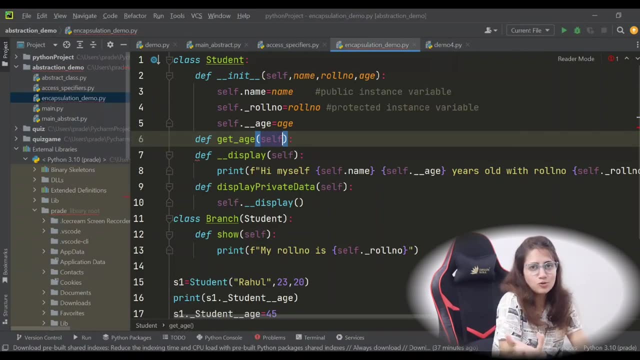 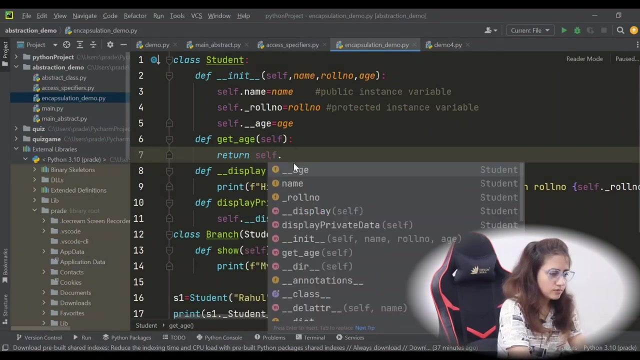 get the age. so just define uh, this name, get what, get age, right, because age is only private. so we use getters and setters on private attributes only so get age and get means to get at the age. so return just self dot, underscore, underscore age, or maybe directly: 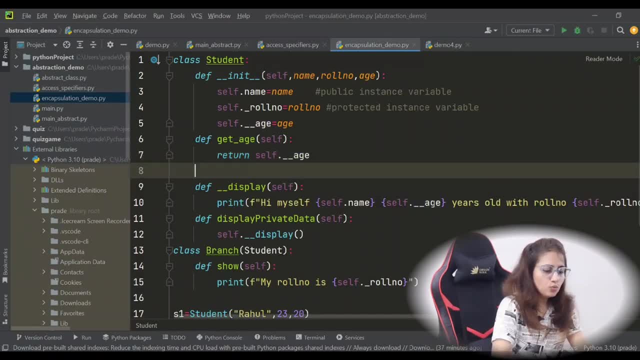 you can print that my age is this and if you want to modify this age, then use setters method like set. it's not like that. you have to give the name getter and setter, just indicate get and set like and just. you can say underscore and the name get and set and then you can use get and set and. 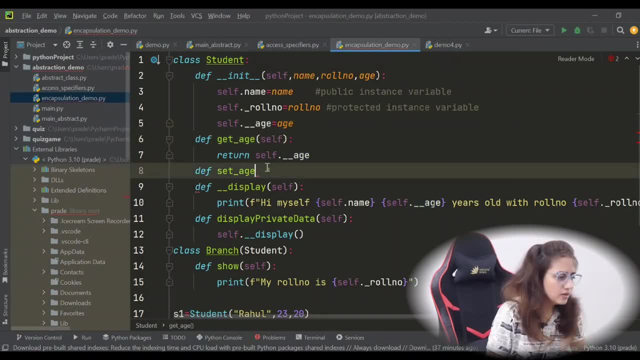 of the attribute name anything you can give right, set age. so i want to modify it so obviously, when we call this function, we are going to provide our age, so let's just maybe number or any parameter name. you can take age, you can take even age, you can take a, you can take xyz, anything right so and 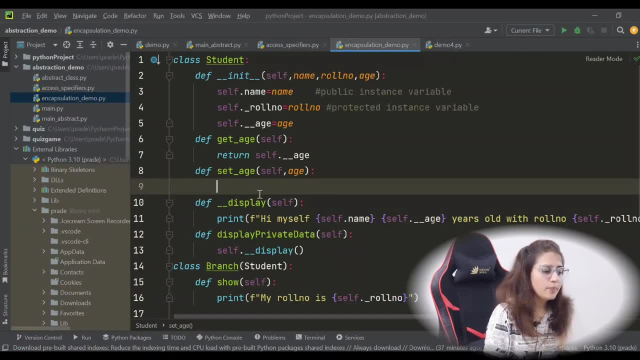 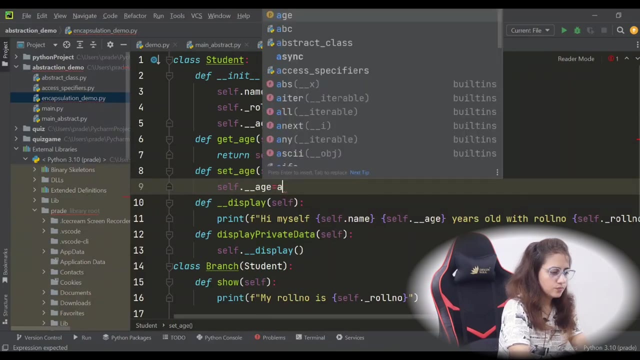 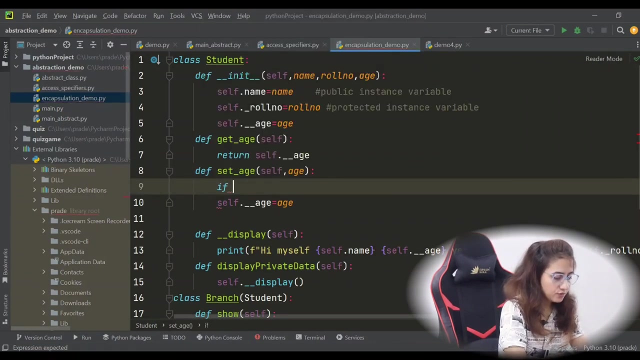 basically setter and getter we use when we uh want to apply some validation logic when we are modifying the age right. so if you want to apply some validation logic, either directly you can set like self dot underscore. underscore age is equal to directly the attribute name age. this is also fine if you want to apply some logic, validation logic, like if this age 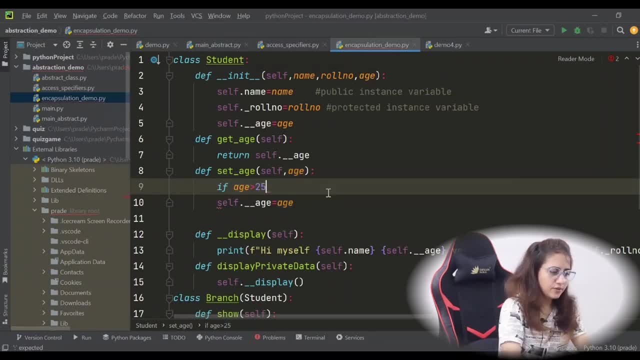 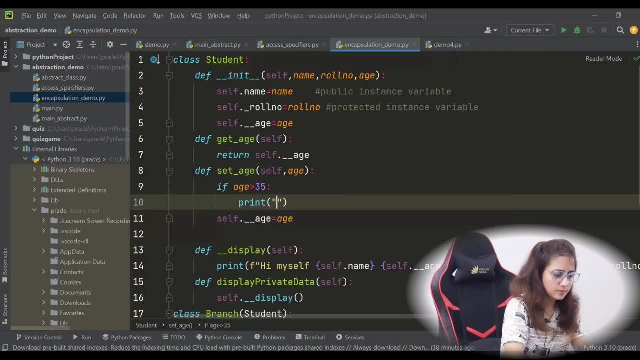 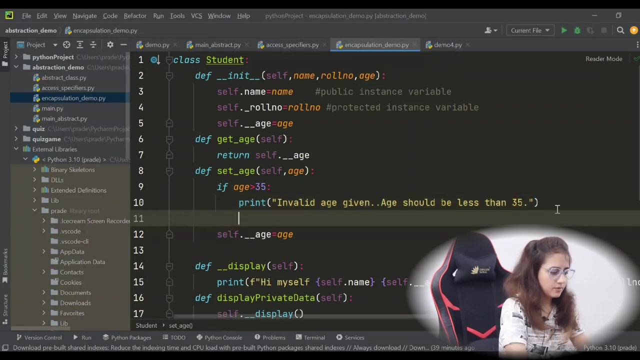 you have given is greater than 25 or greater than, suppose, 35, then print, suppose i have some restriction- a should be less than 35, so if greater than 35, then it will give error, else set the age, else just set age right now, suppose let's just comment out. 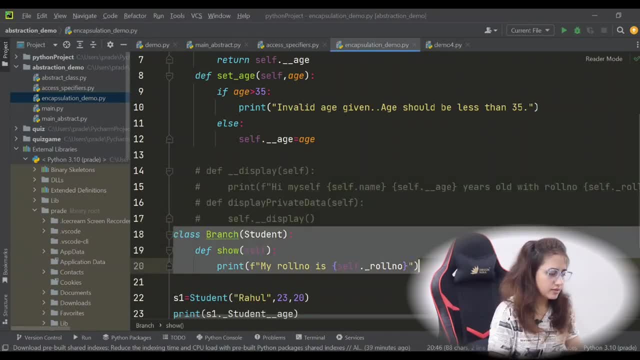 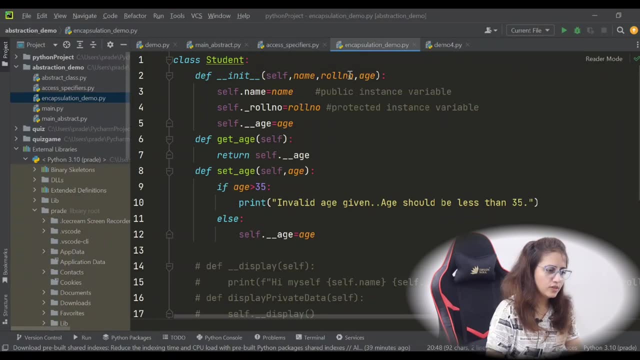 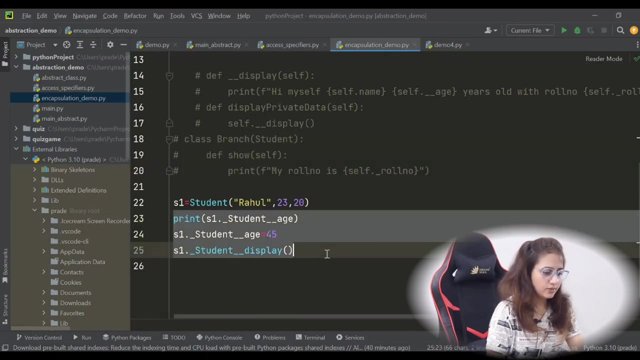 these two methods and comment out this class as well. derived class. now let's create s1 student. what you need to pass name roll number age- okay, name roll number age- and now use get and set method. so if you want to get the age, just call s1 dot. 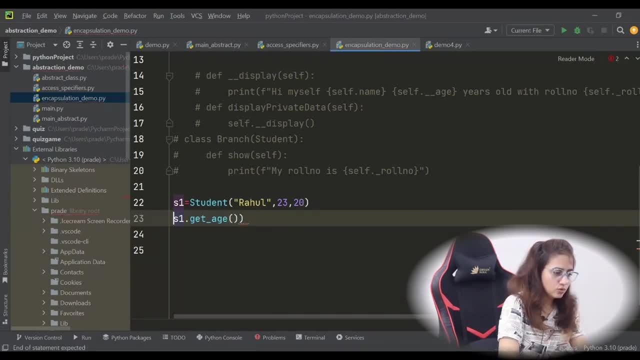 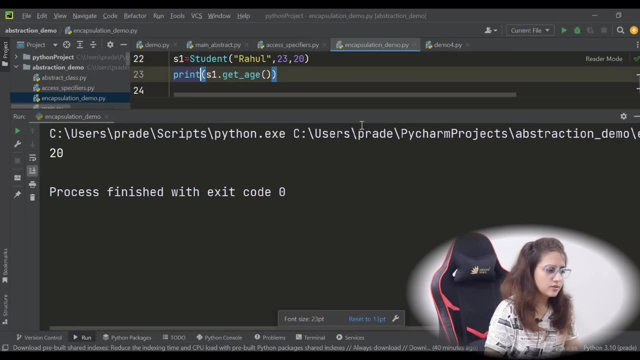 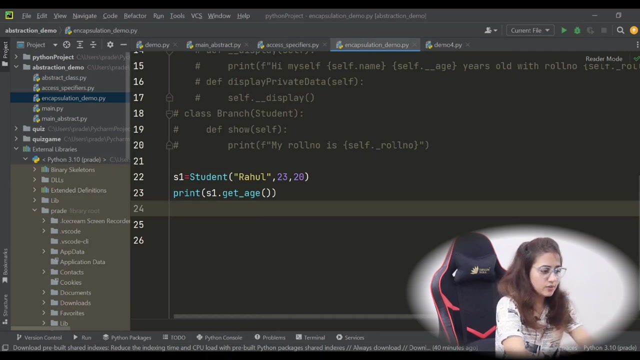 get age and it is returning. so definitely you have to print. let's run this and it will print ages 20.. okay, if you want to modify that private variable, private attribute age, then just call set age and here just i just want to pass like 34, maybe, okay, and after that just again i want to print. 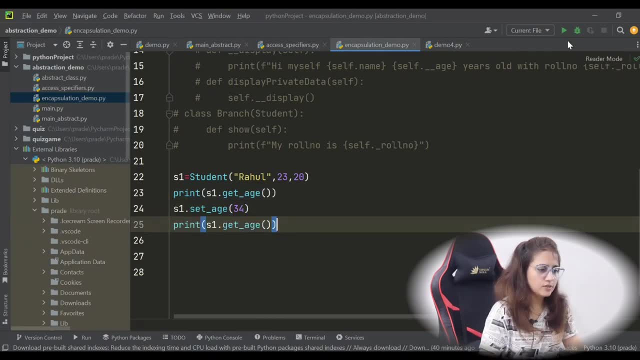 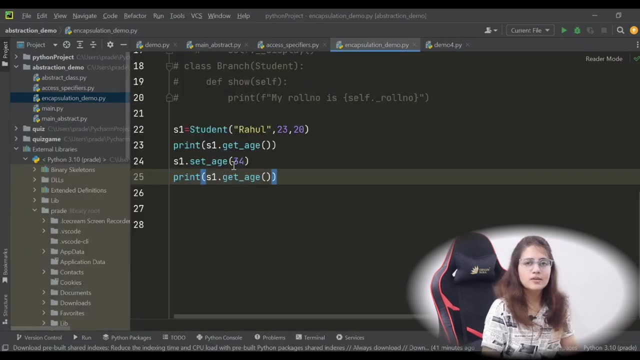 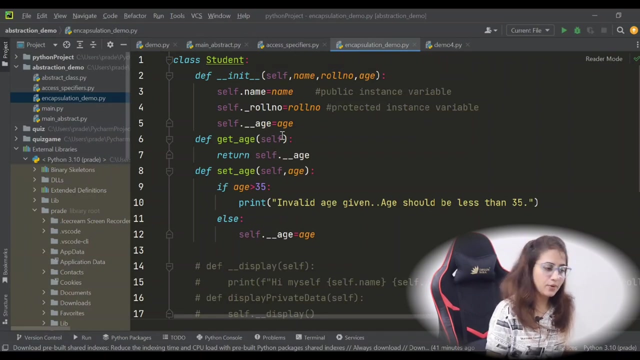 age. just copy paste this thing and let's run this. see, first it was 20, then it was 34, using getters and setters method. it's a good idea. it's a good practice to do that. and another thing is in writing. Herman said there are so many different methods to modify.